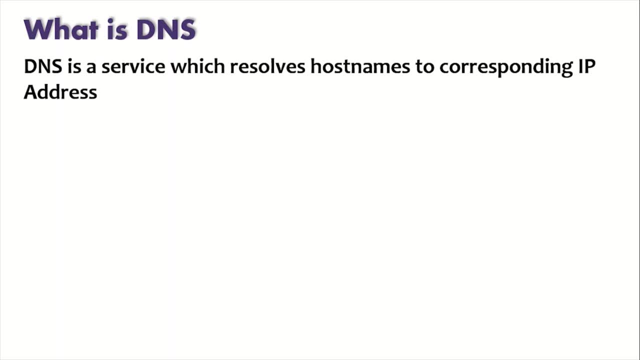 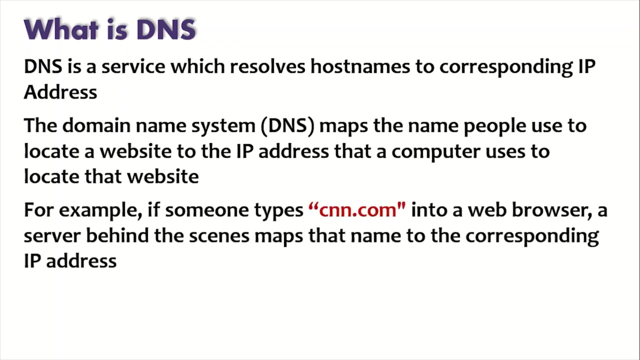 host name to corresponding IP address. So what is it all about? So the domain naming system, or DNS, maps the name people used to locate a website to the corresponding IP addresses of that particular website. Let's say, for example, if someone is typing cnncom into a browser, the server behind 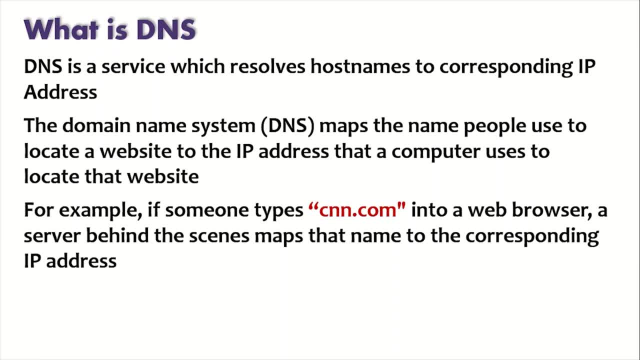 the scene maps that name to the corresponding IP address. So let's say, for example, if someone is typing cnncom into a browser, the server behind the scene maps that name to the corresponding IP address. So the IP address looks say somewhat like this. The structure of the IP address might 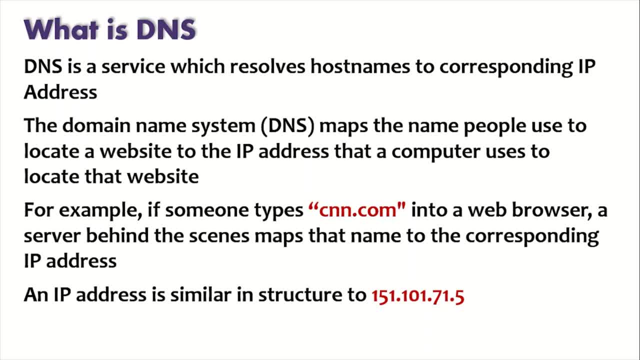 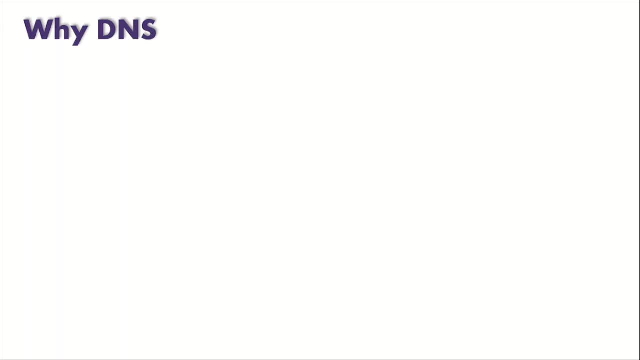 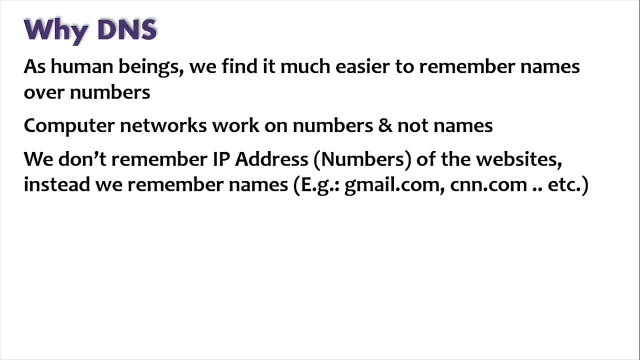 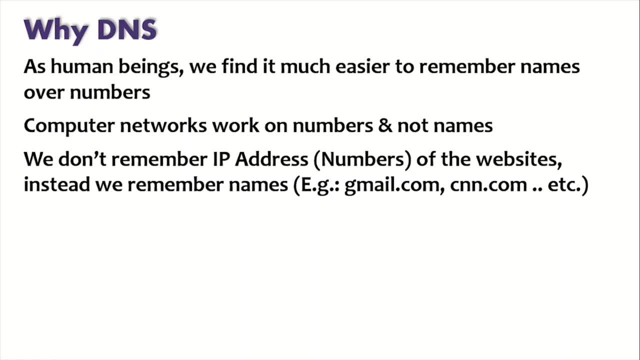 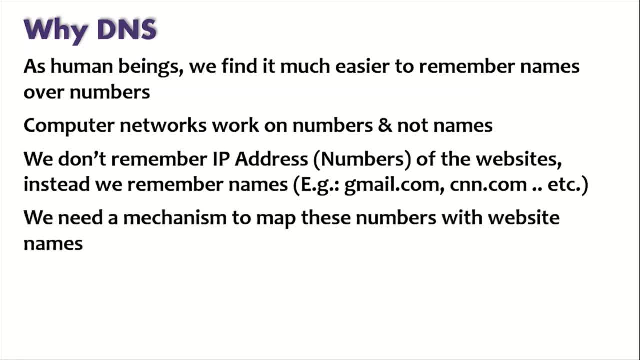 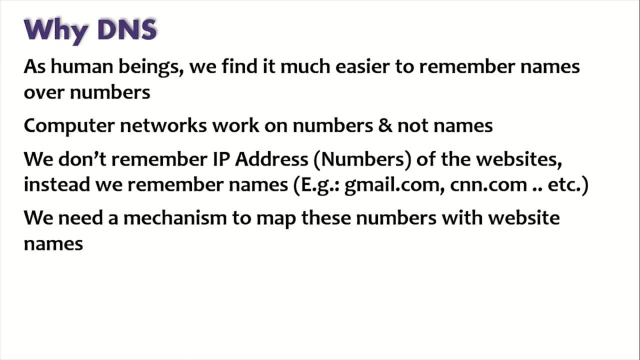 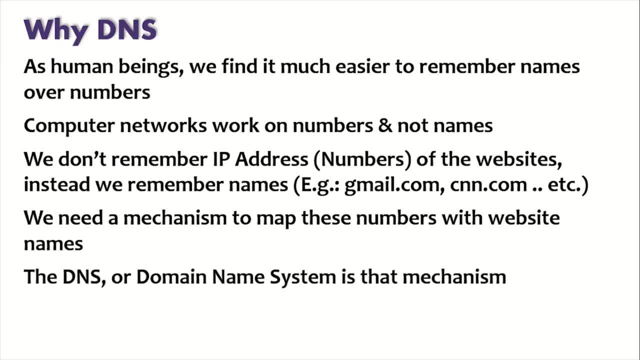 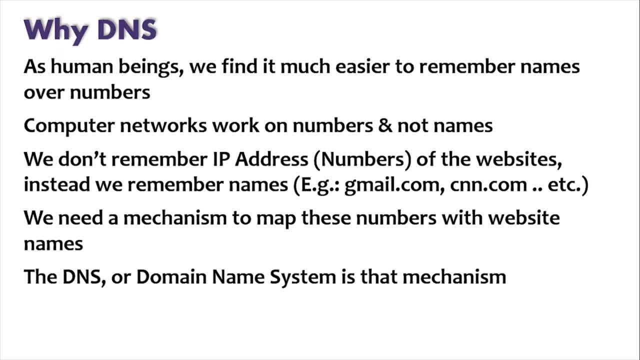 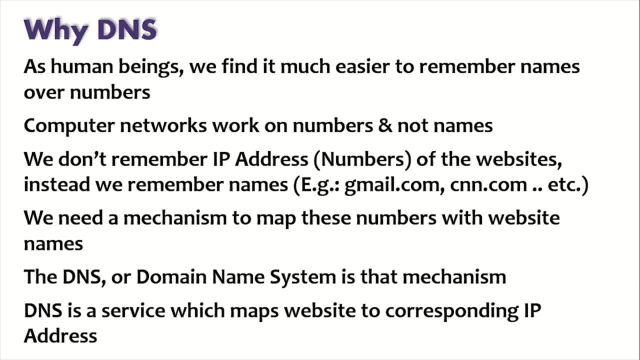 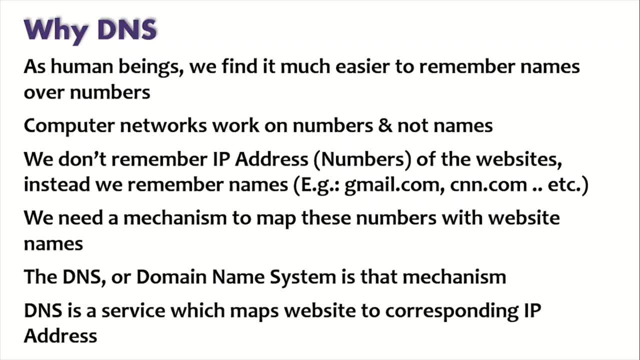 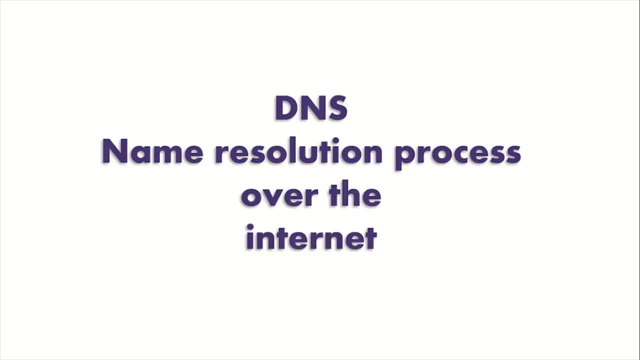 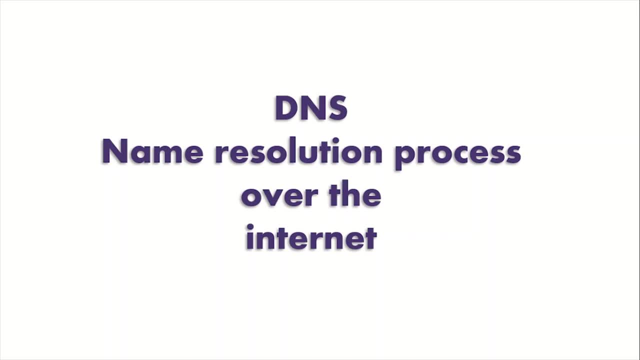 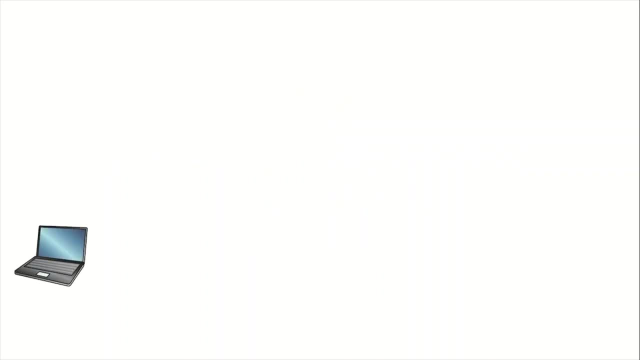 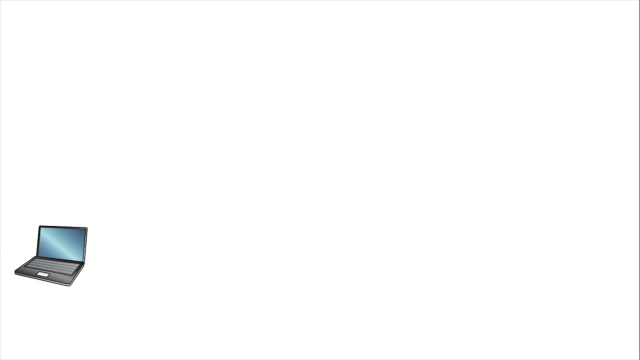 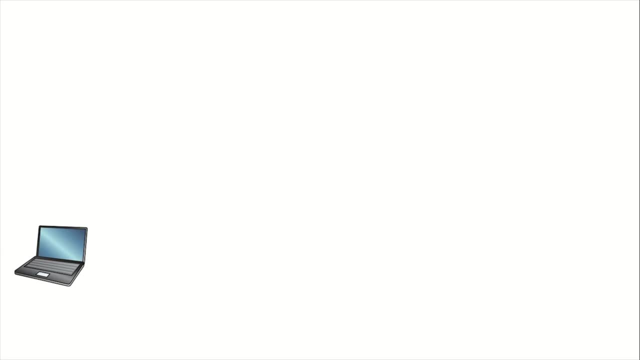 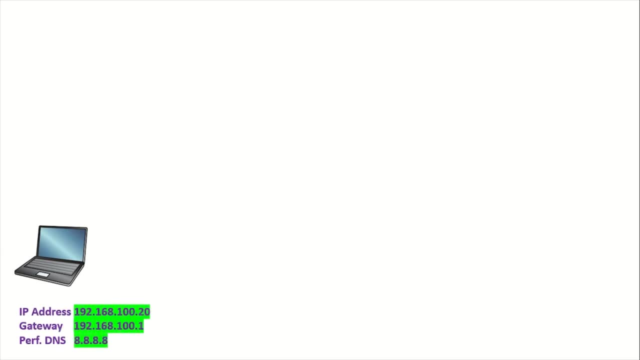 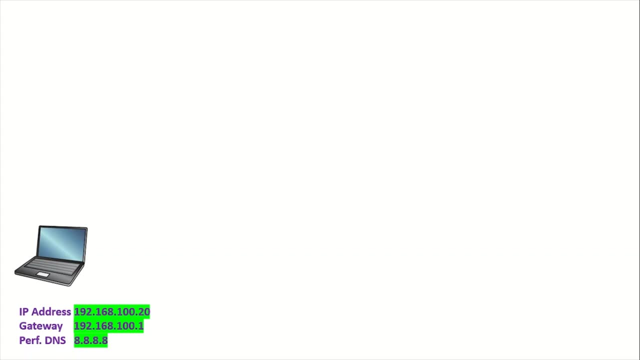 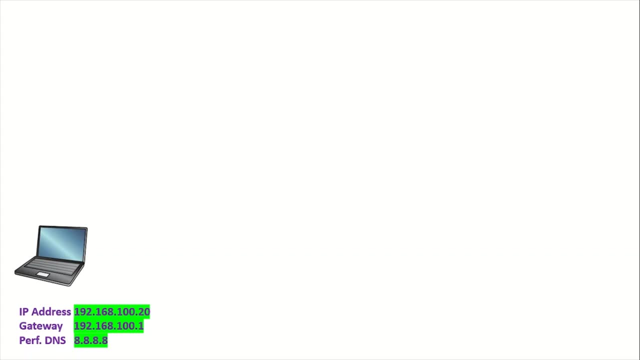 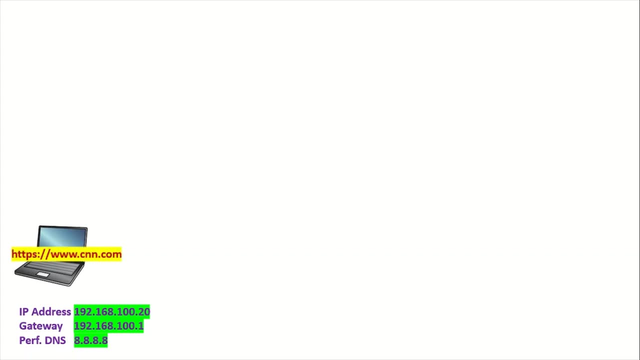 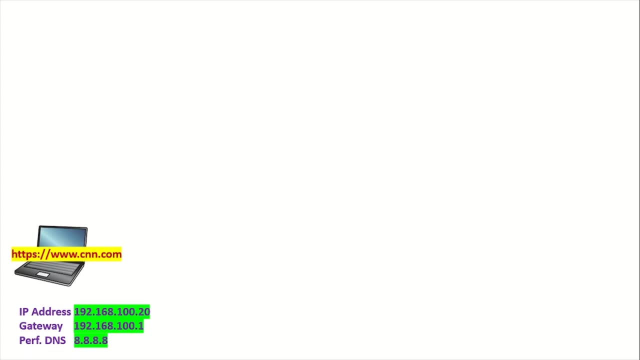 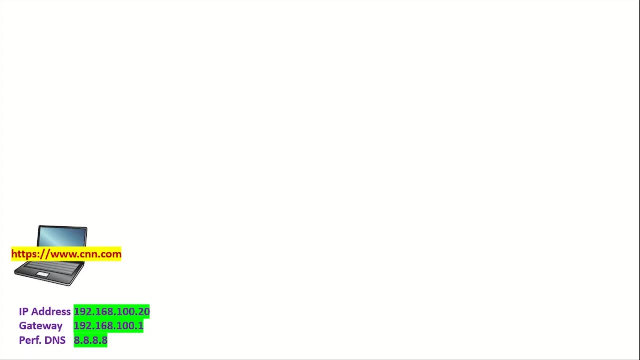 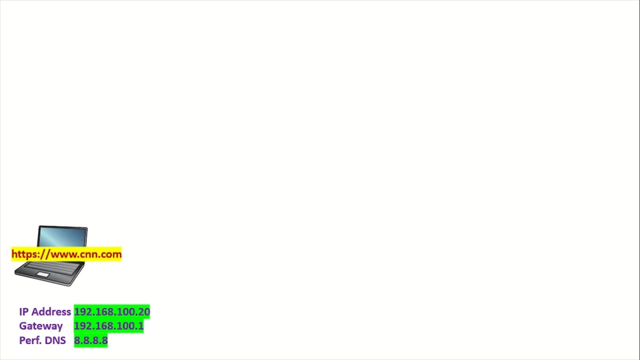 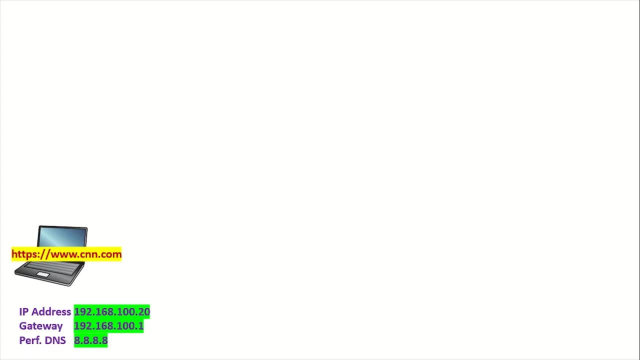 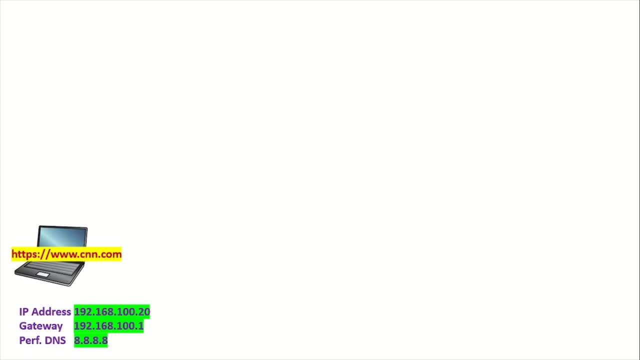 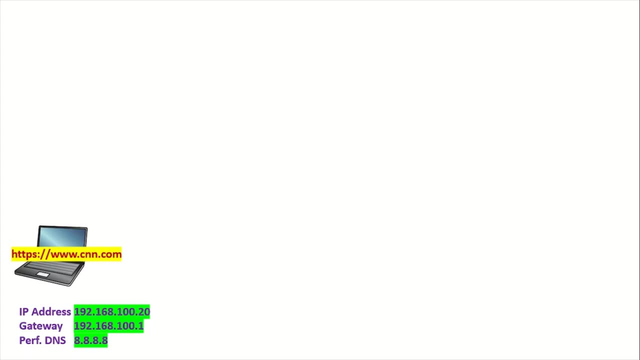 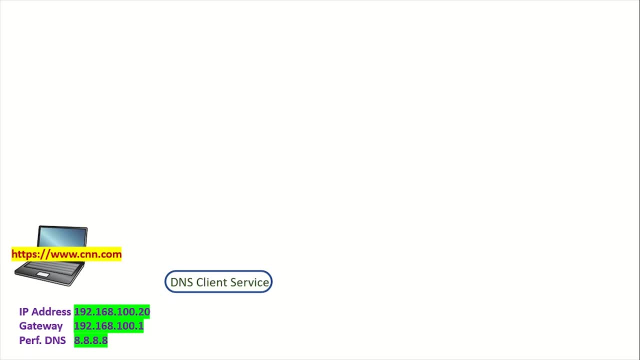 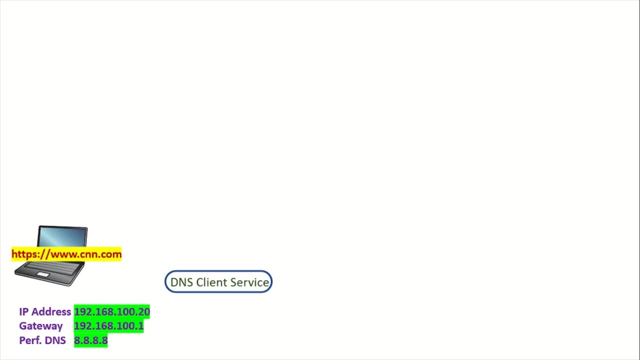 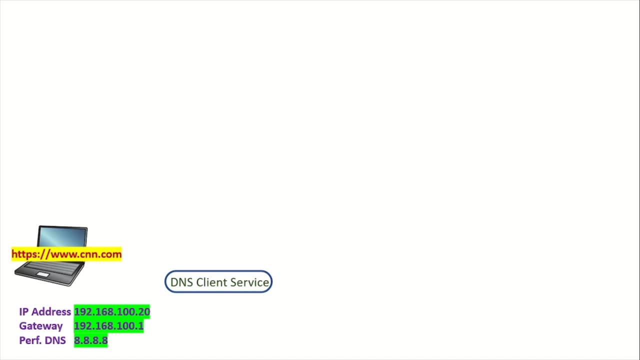 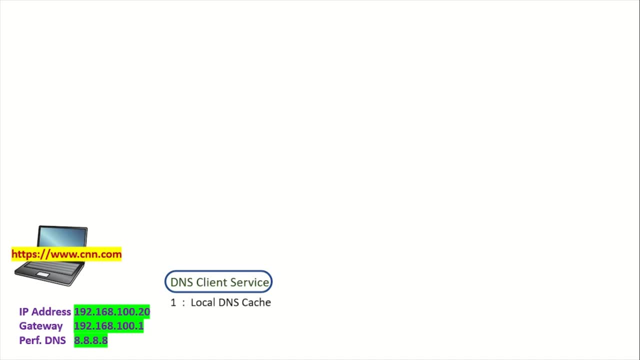 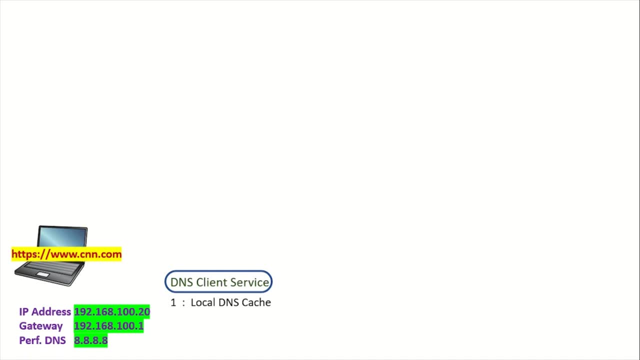 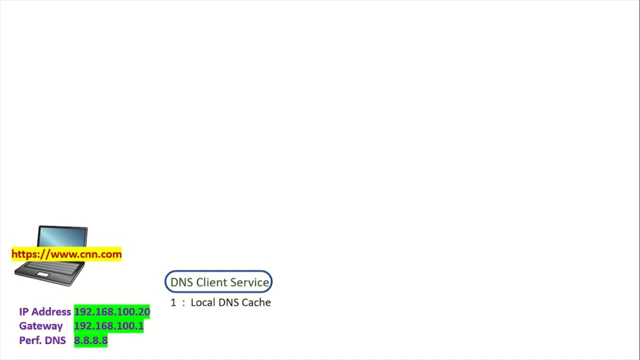 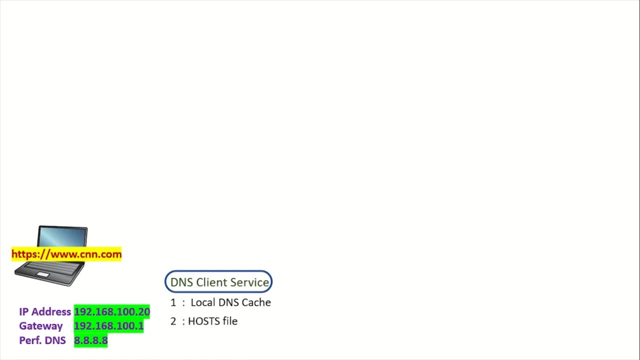 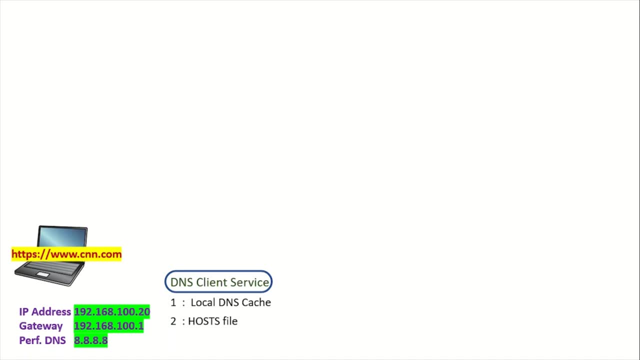 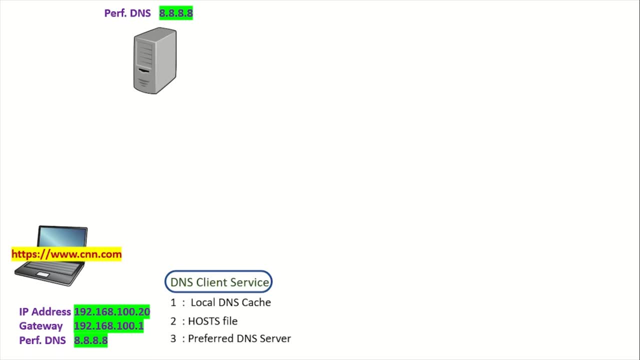 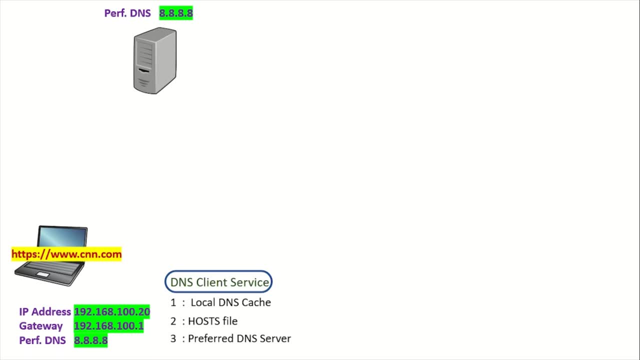 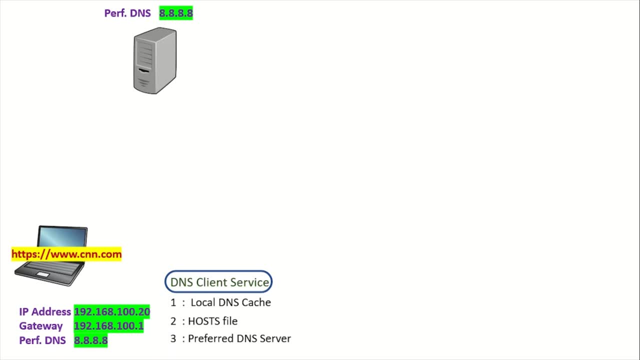 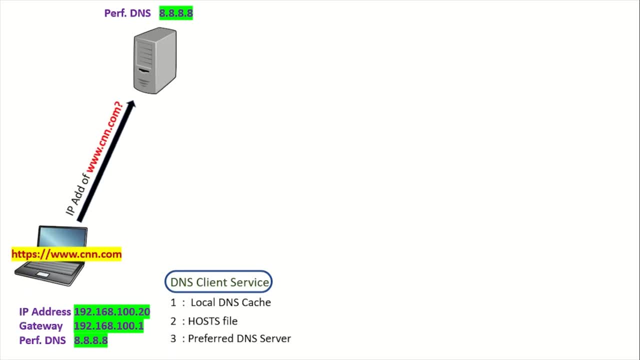 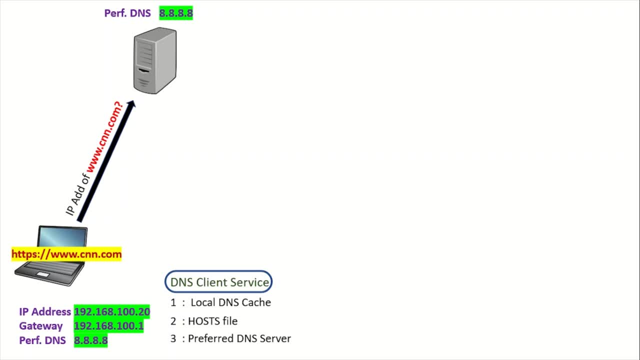 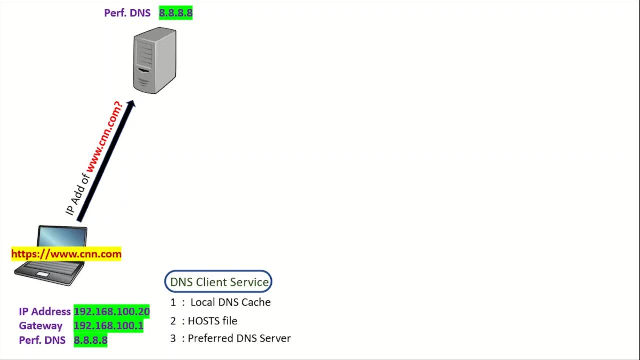 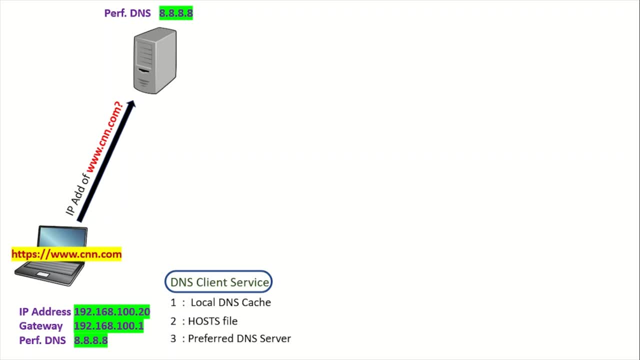 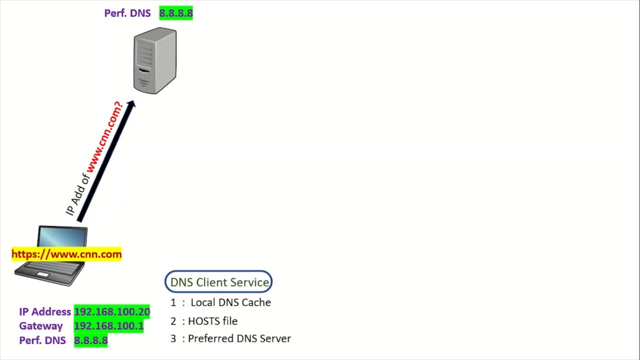 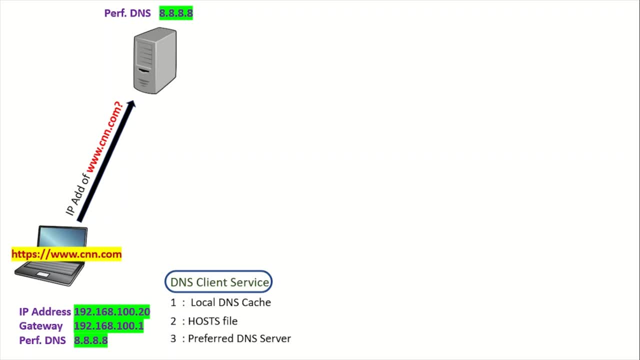 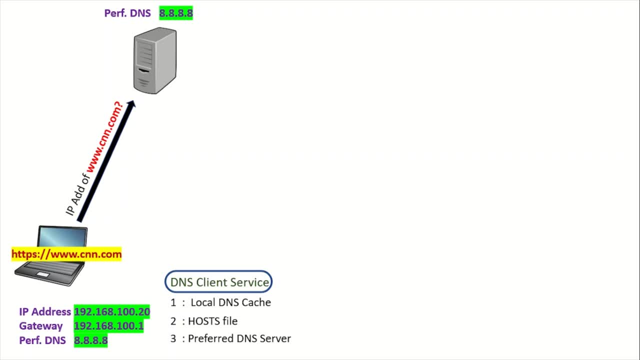 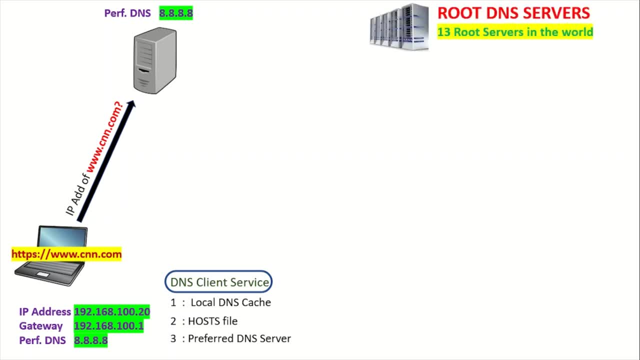 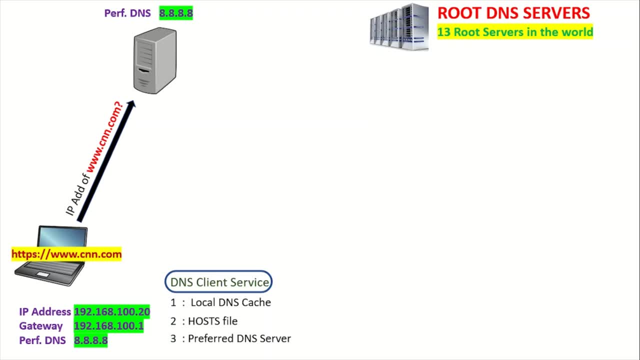 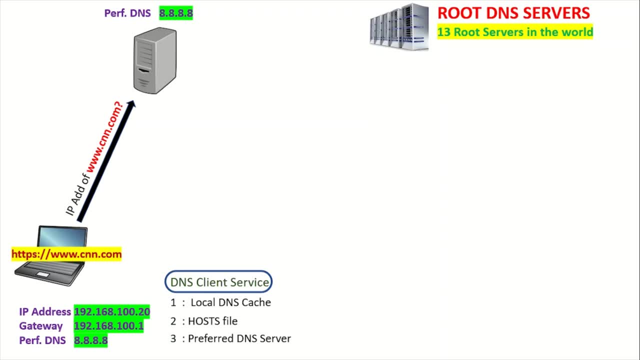 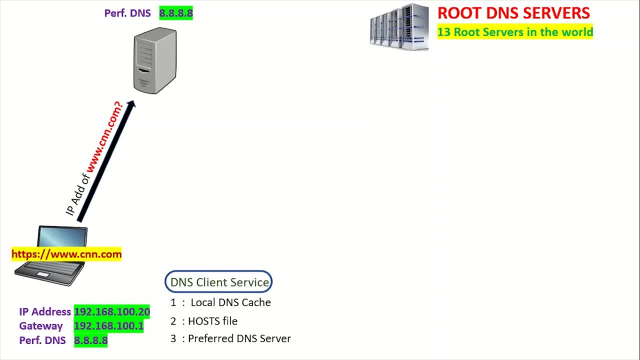 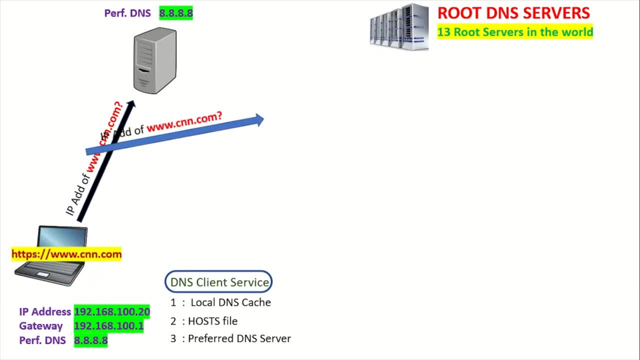 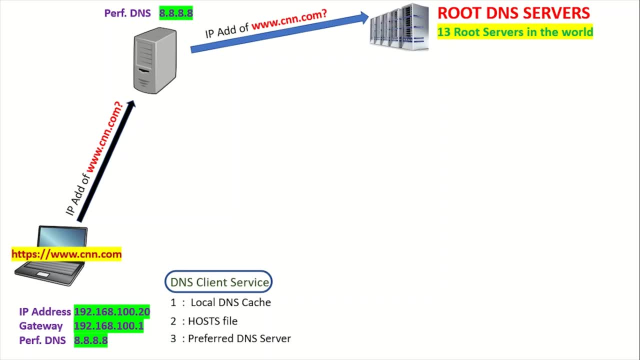 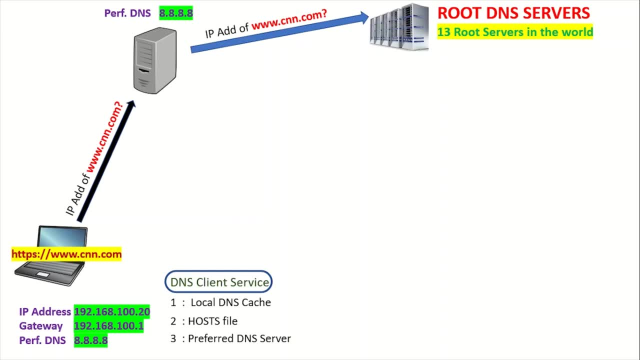 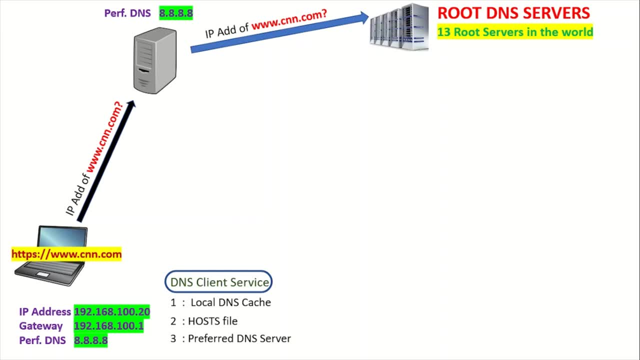 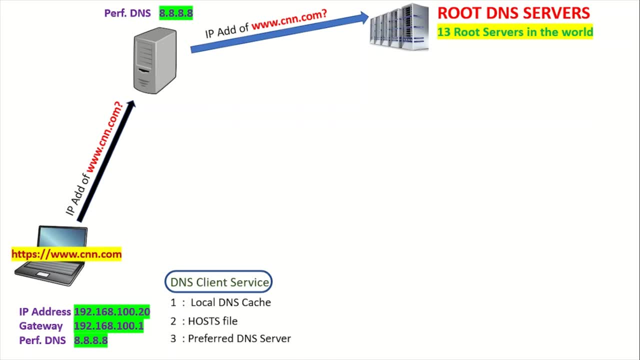 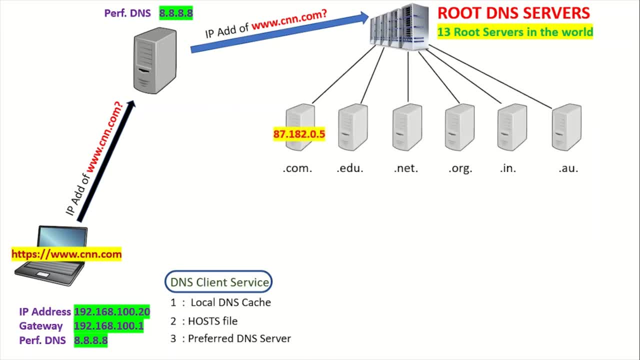 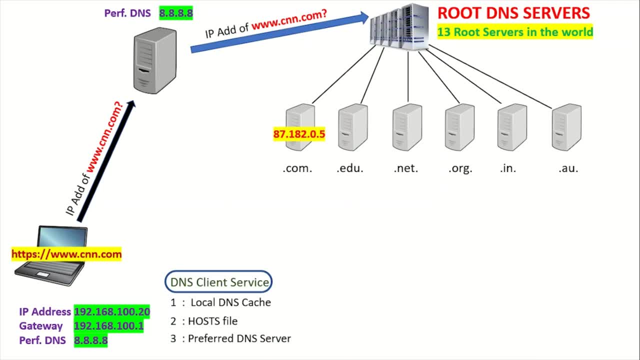 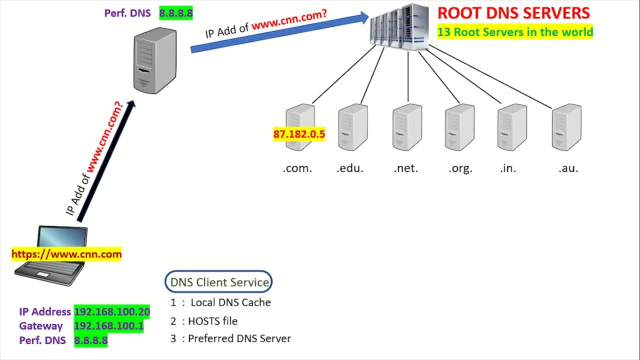 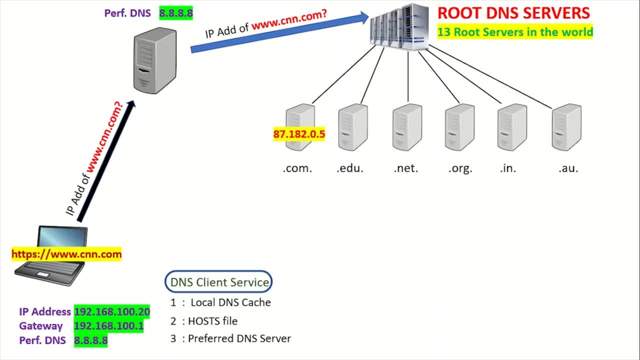 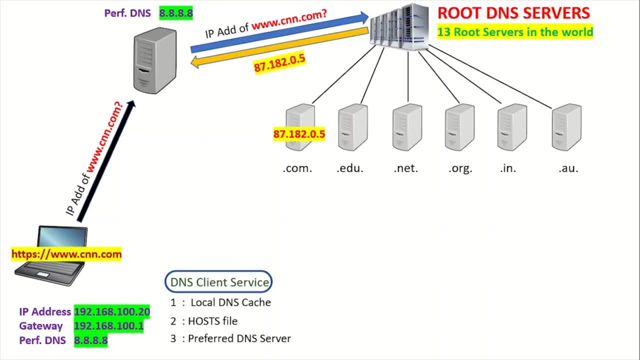 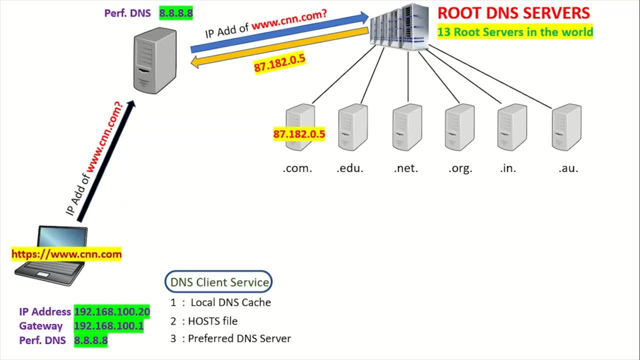 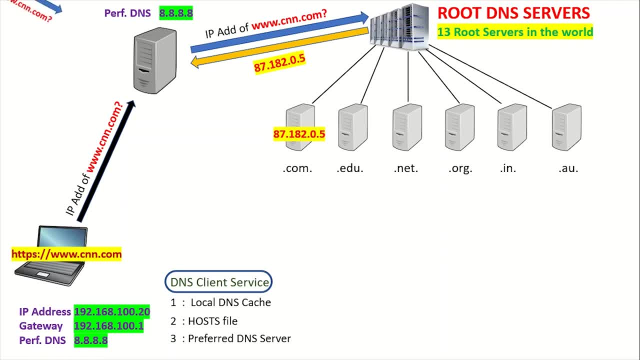 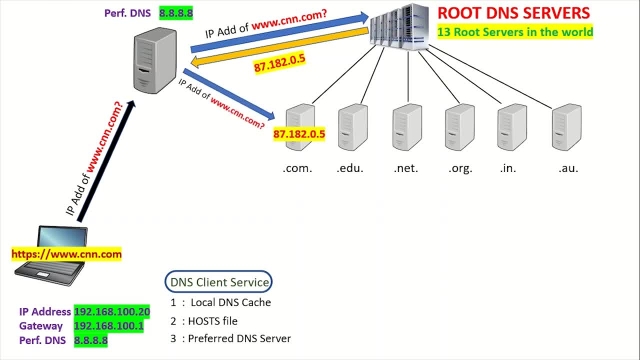 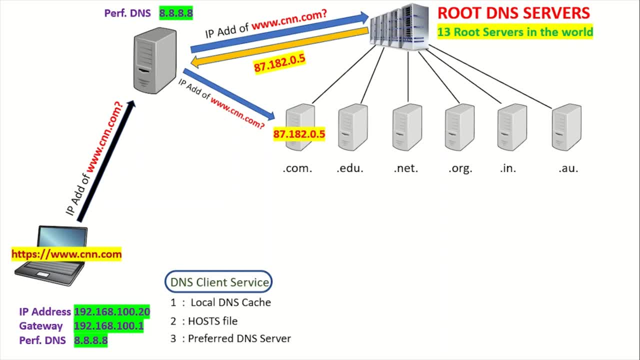 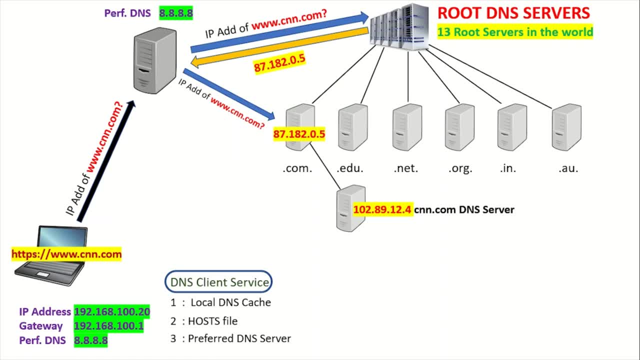 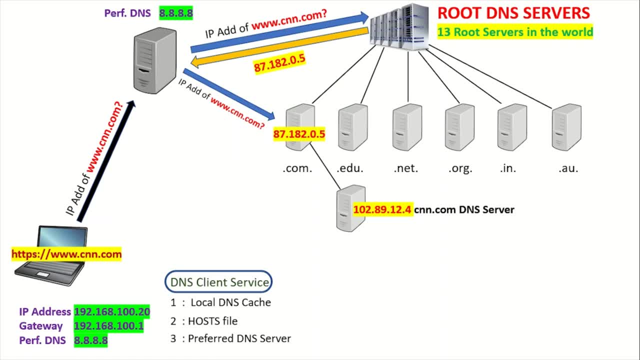 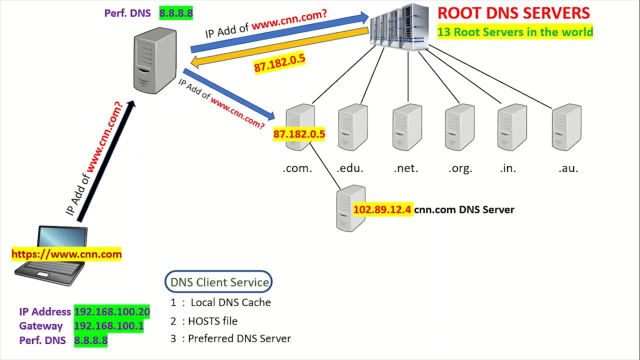 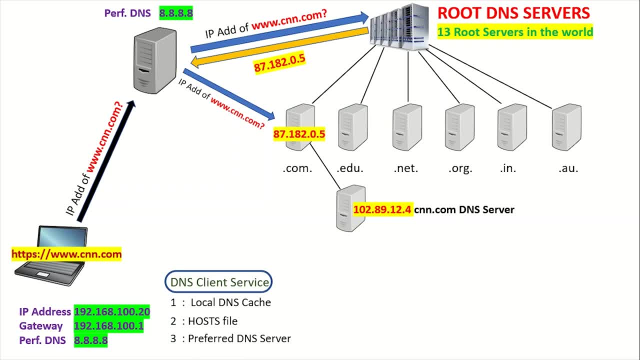 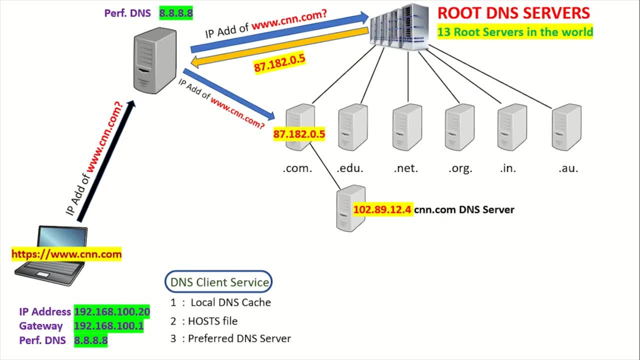 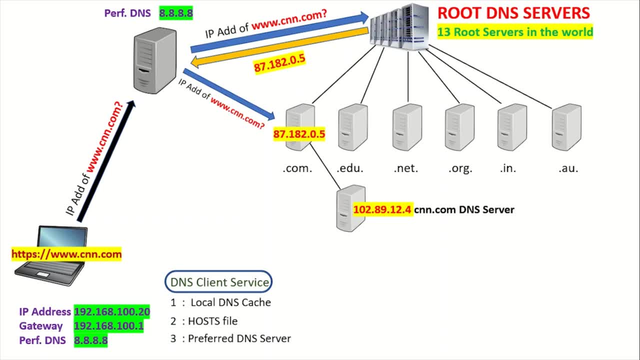 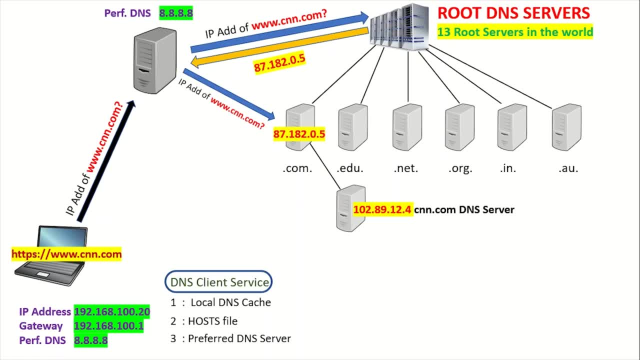 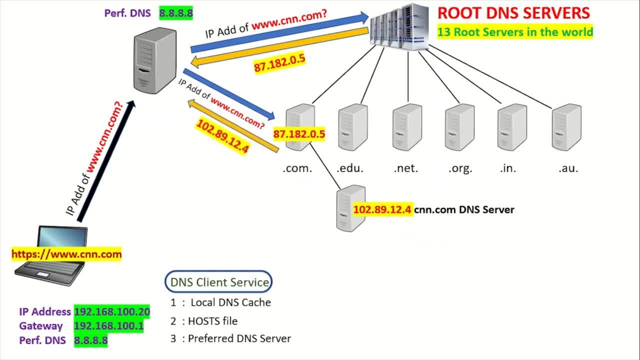 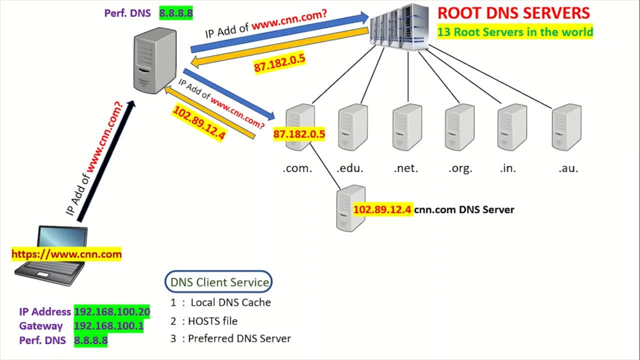 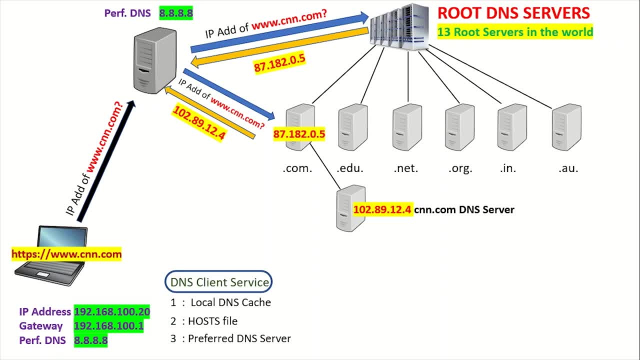 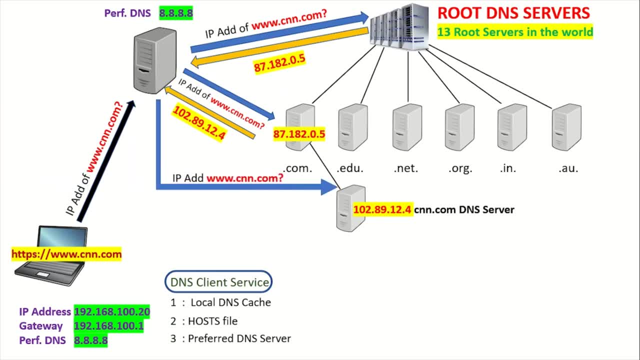 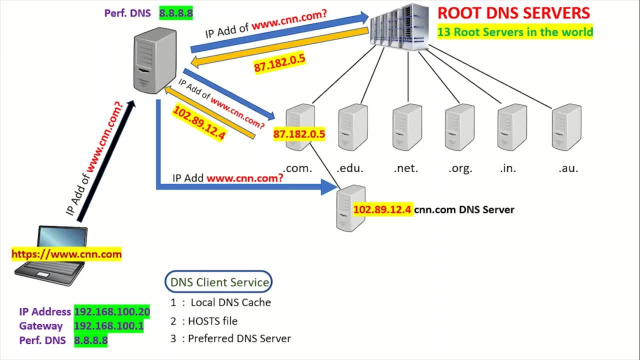 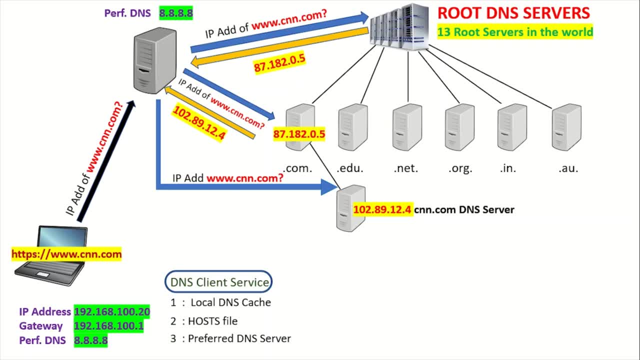 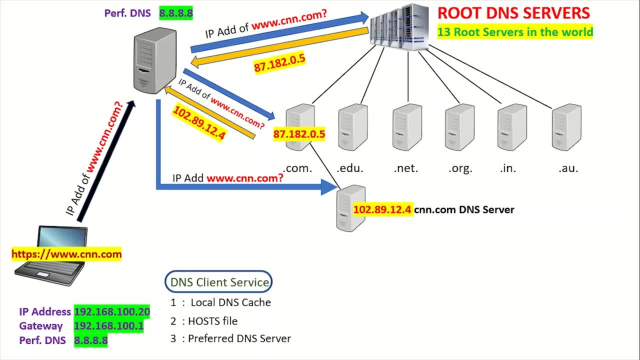 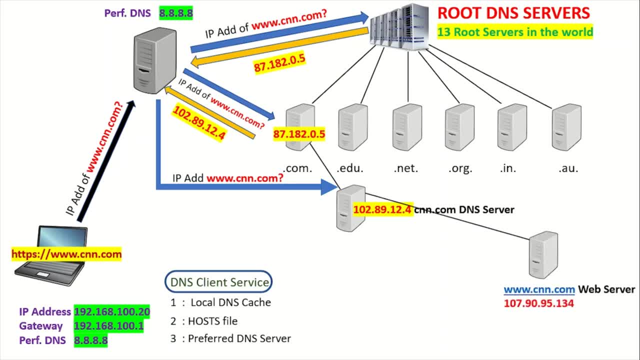 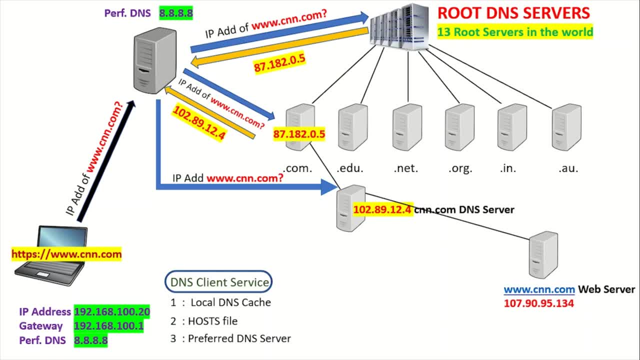 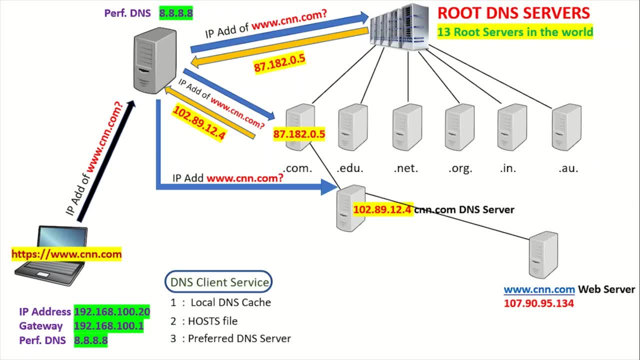 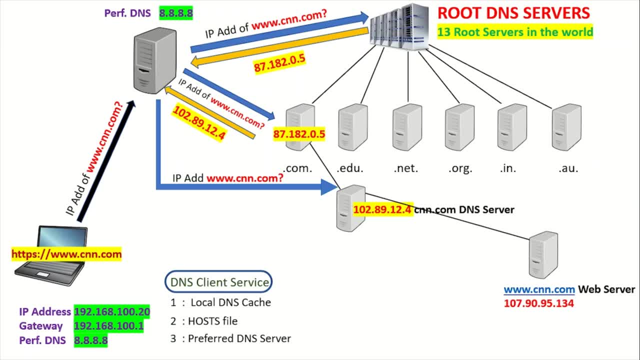 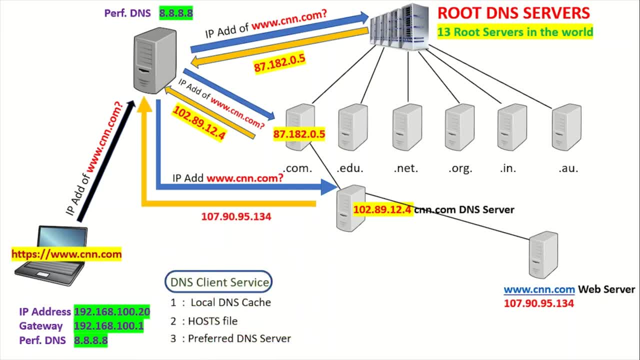 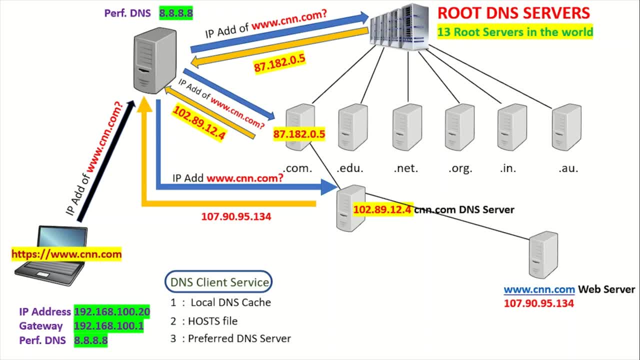 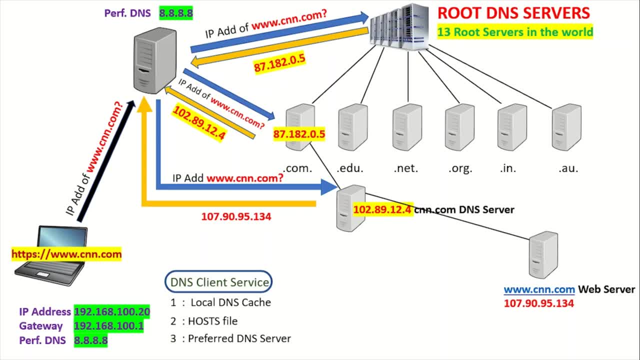 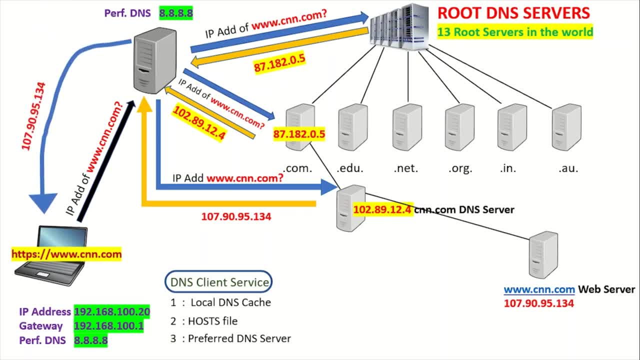 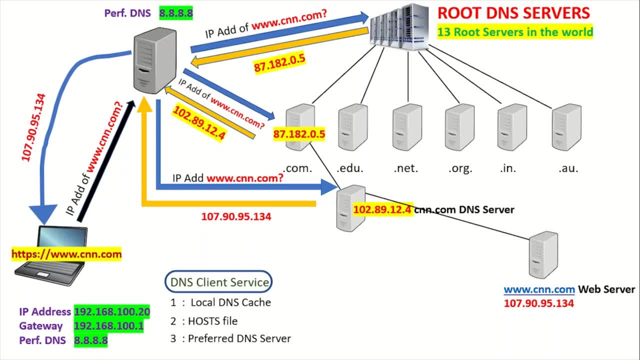 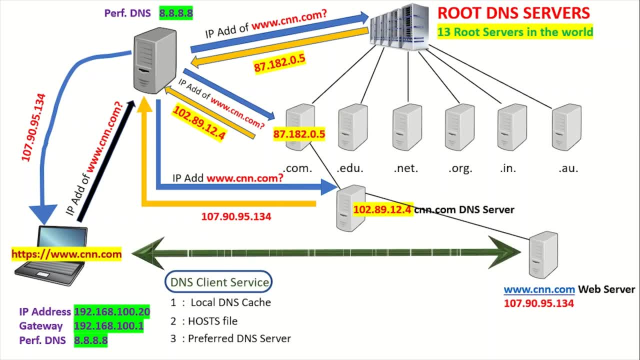 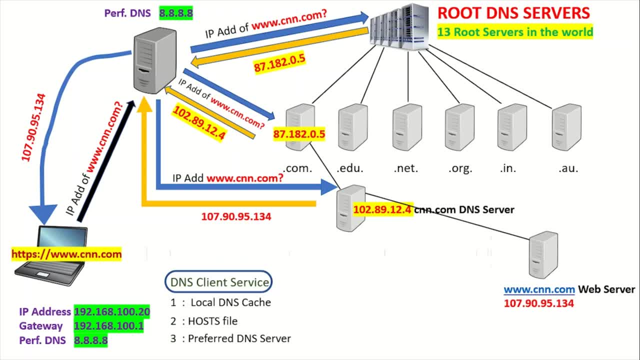 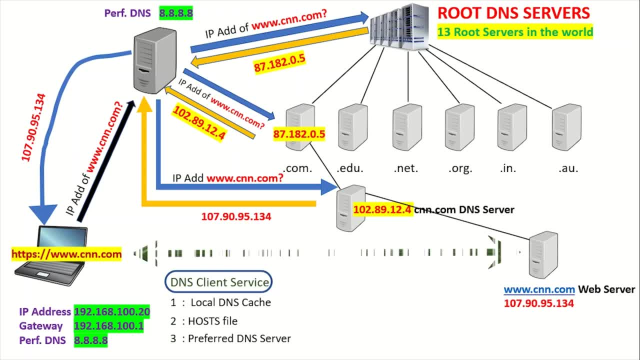 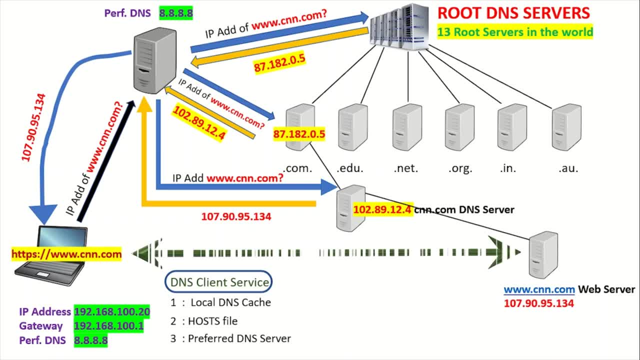 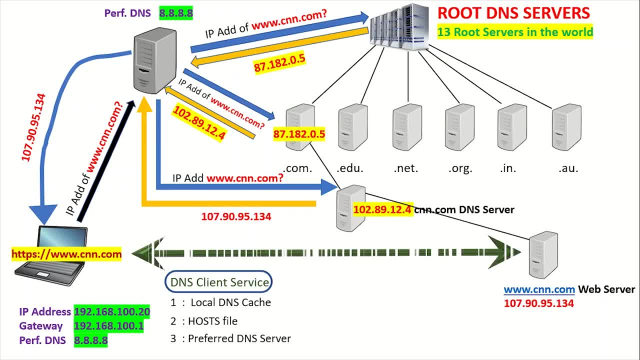 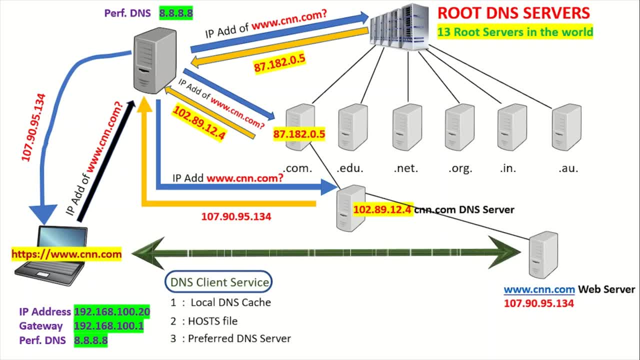 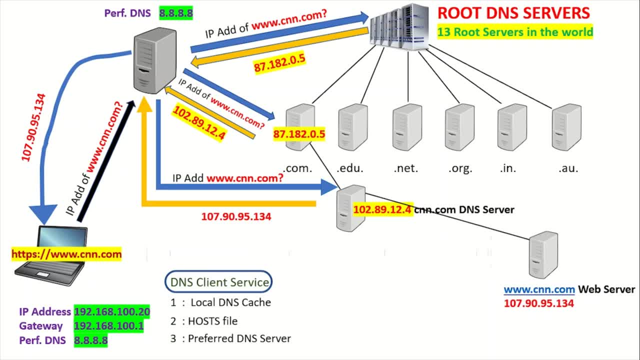 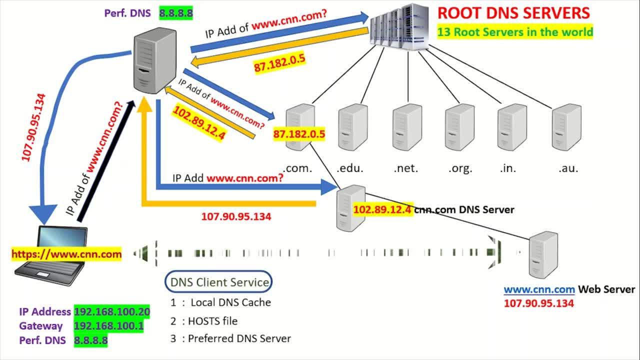 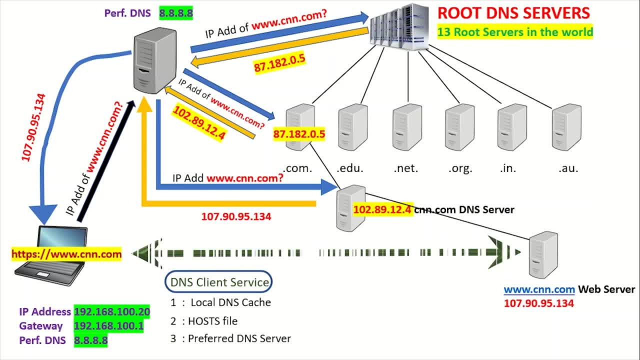 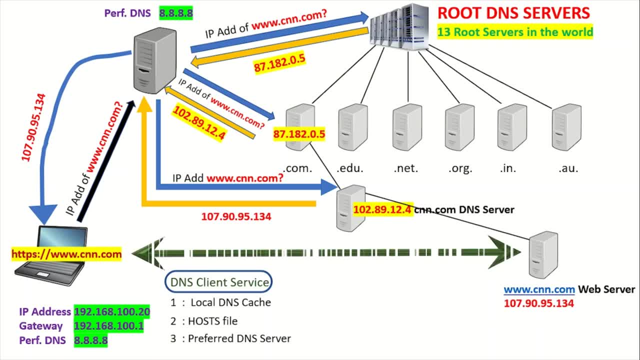 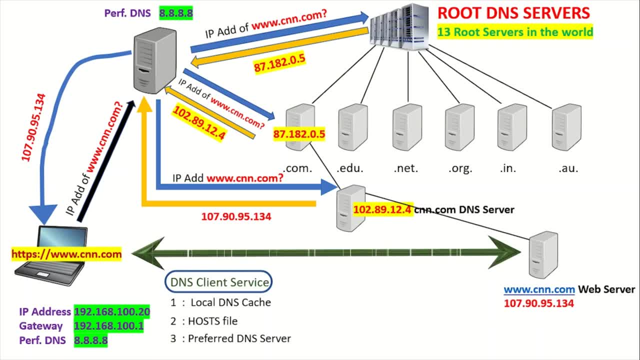 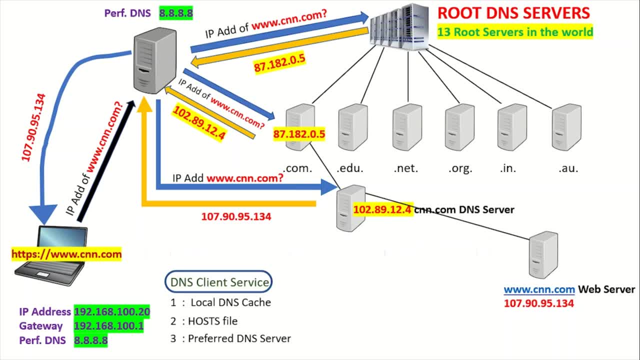 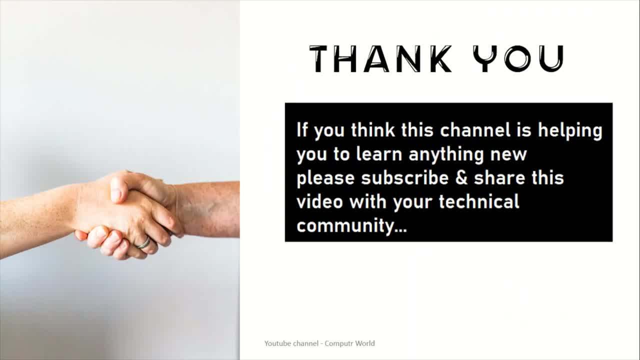 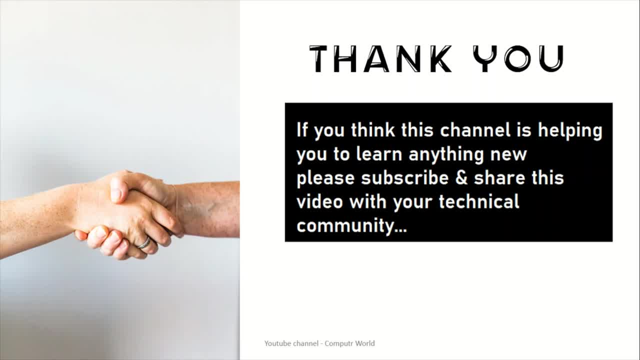 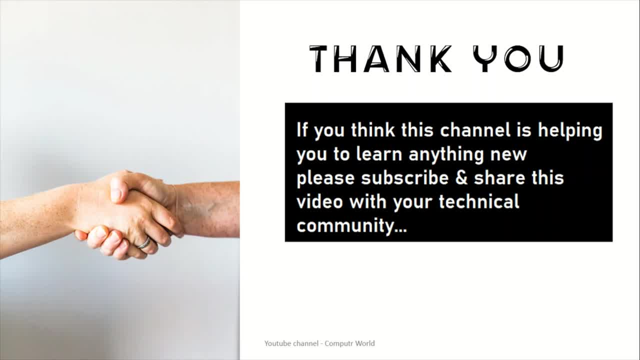 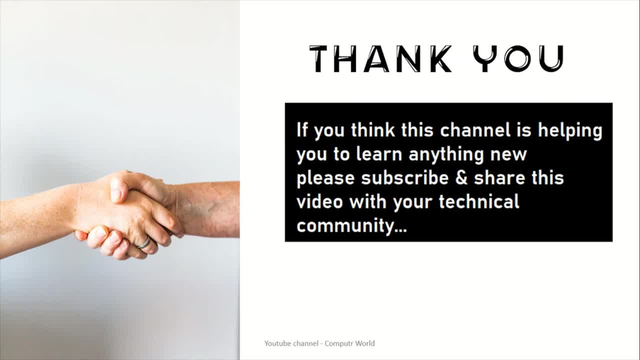 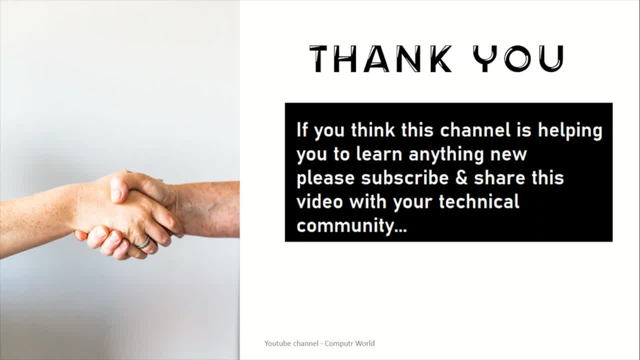 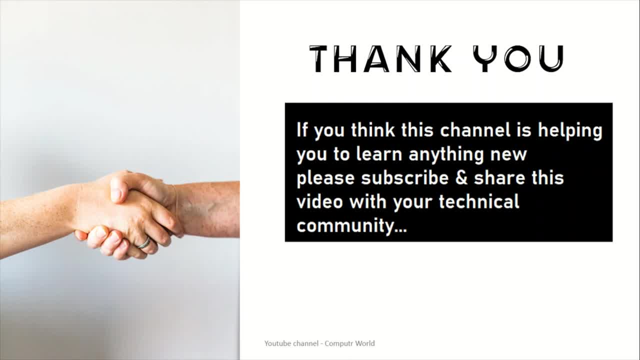 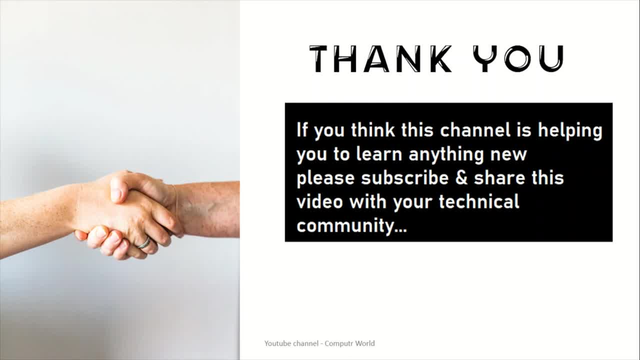 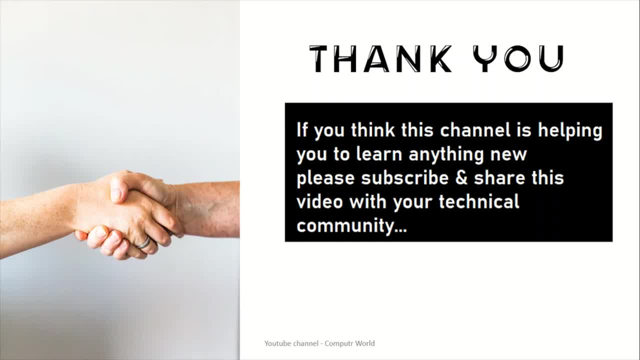